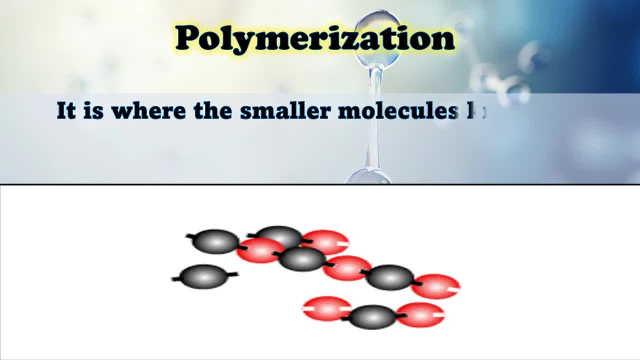 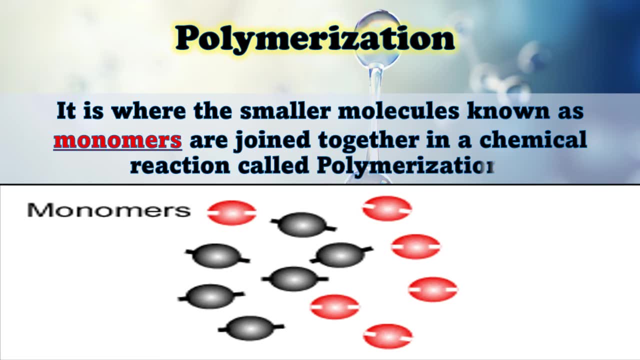 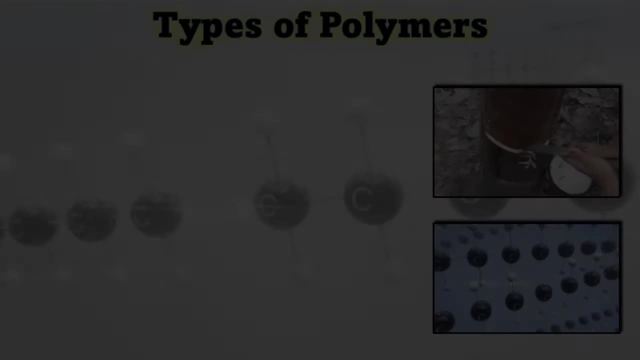 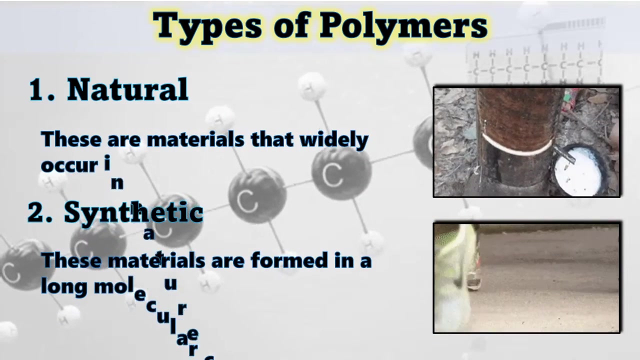 These smaller molecules are known as monomers. Hundreds of thousands or even millions of monomers are joined together in a chemical reaction known as polymerization. Some polymers are natural, while the rest are synthetic. Natural polymers are rubber, proteins and DNA. 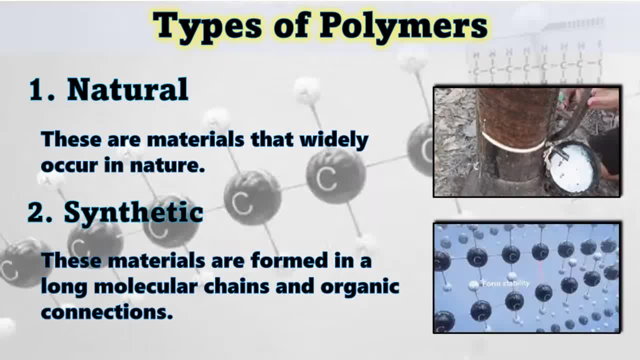 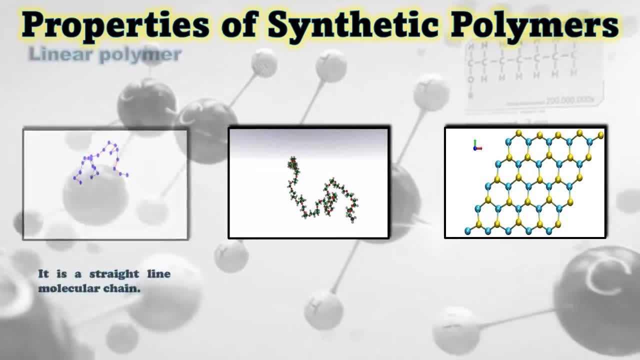 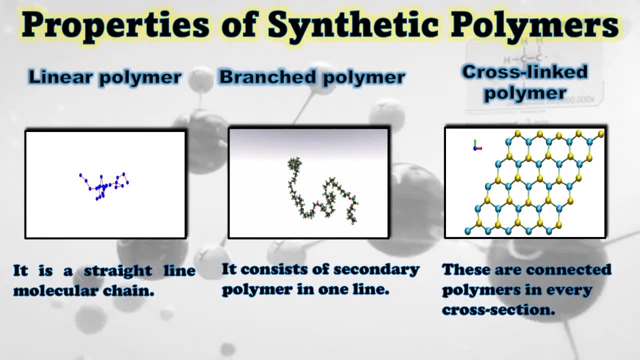 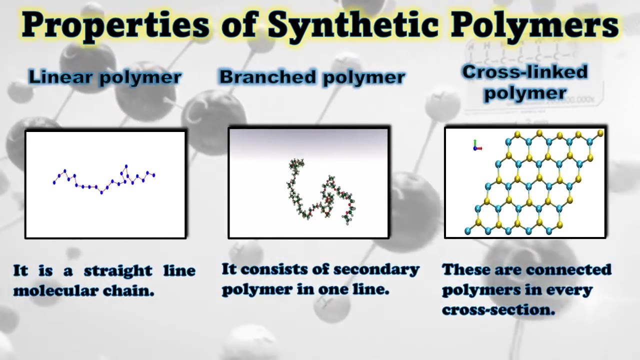 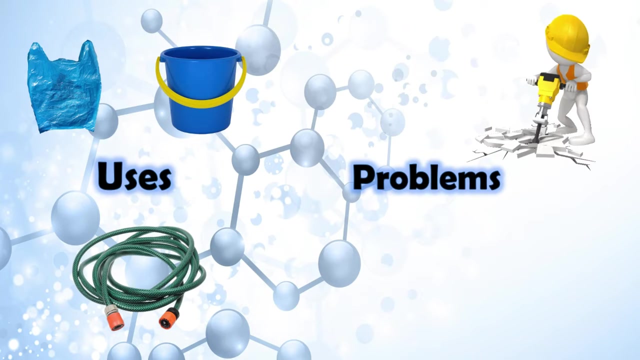 Synthetic, on the other hand, are plastics. The properties of polymer depend on its structure. We have linear polymer, branch polymer and cross-linked polymer. Unlike cross-linked polymers, the first two structures can be reshaped upon heating. Plastic bag, bucket and hose are good examples of synthetic polymers. 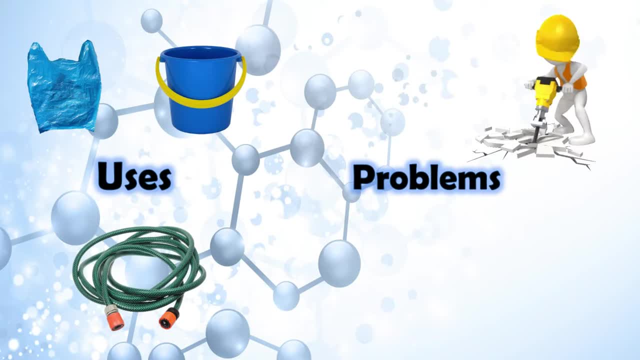 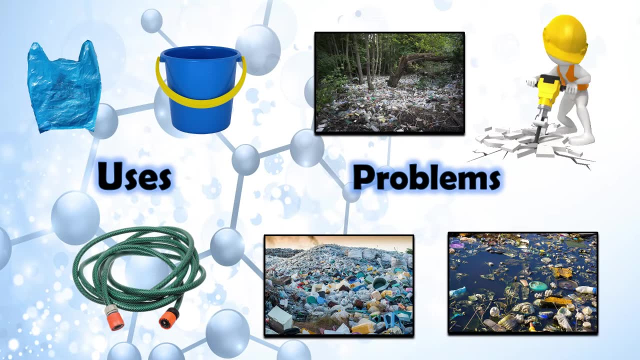 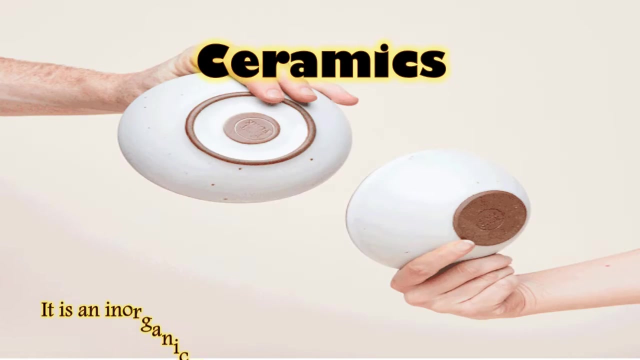 But do you know that there is a major problem of using these things? Exactly, That is pollution. However, we can still reduce, reuse and recycle these things. Oh, that sounds great. Next, we have ceramics. It is an inorganic, non-metallic solids that has been shaped and then homogenized. 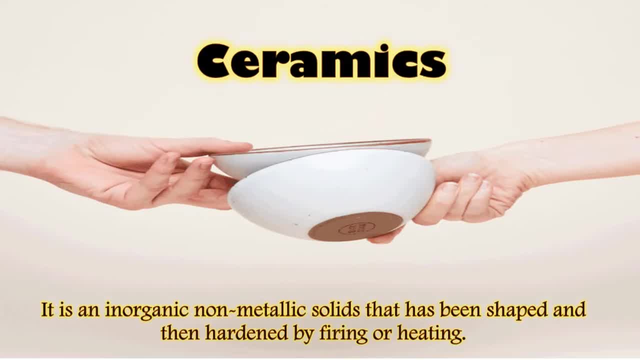 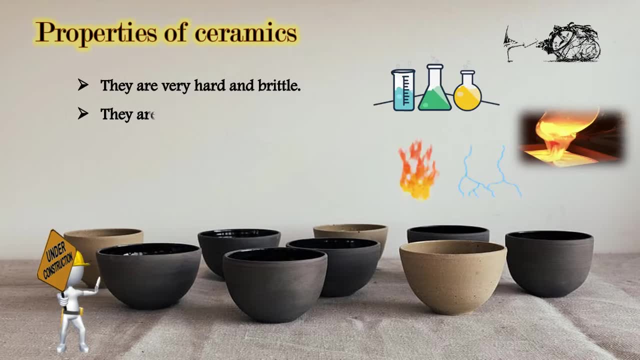 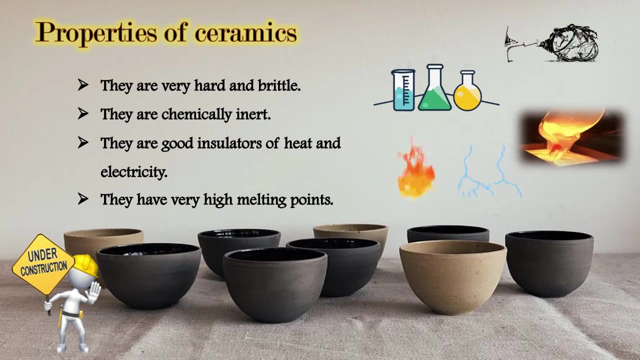 They can be hardened by firing or heating. Ceramics are very hard and brittle, chemically inert, good insulators of heat and electricity, and they have very high melting points. These special properties make them useful in our everyday life. Traditional ceramics are clean. 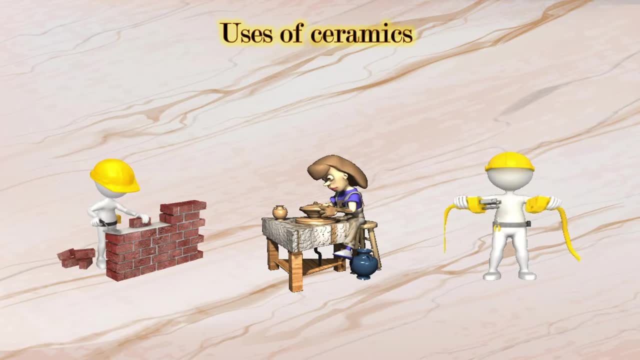 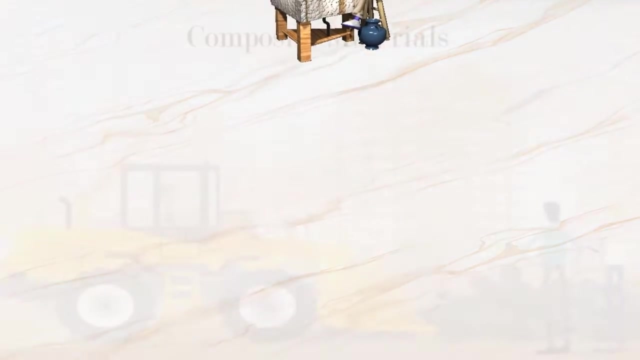 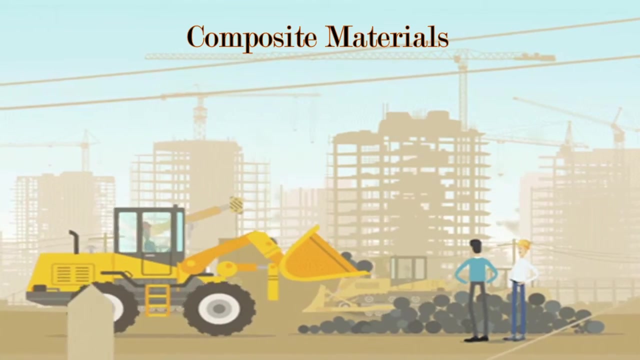 They have a very high melting point. These special properties make them useful in our everyday life. They are clay-based. with some additives. They are very useful as construction materials, decorative items and electrical insulators. That was cool. Do you know that polymers and ceramics are some of the substances used to form a composite material?